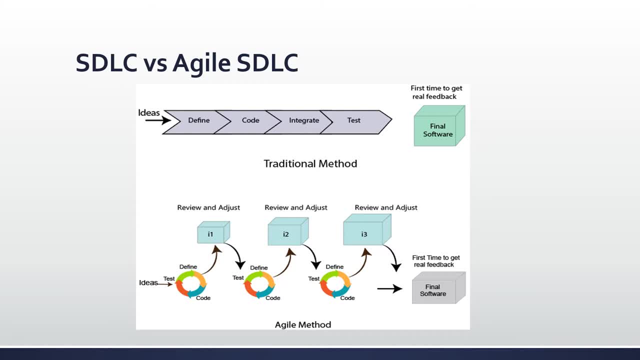 that fulfills the customer requirements within time and cost estimates. Agile software development lifecycle is a combination of both iterative and incremental process models. It focuses on process adaptability and customer satisfaction by rapid delivery of working software product. Agile SDLC breaks down the product into small incremental builds. These builds are provided. 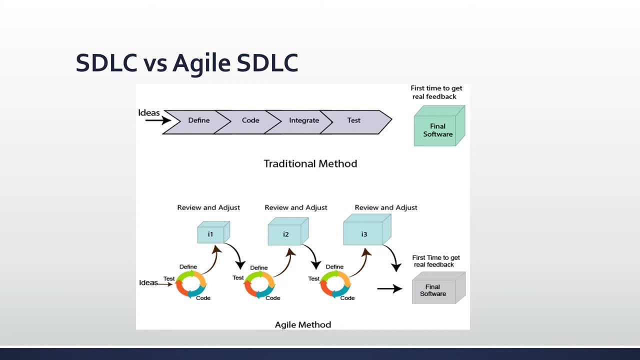 into iterations In the Agile SDLC development process. the customer is able to see the result and understand whether he or she is satisfied with it or not. This is one of the advantages of the Agile SDLC model. One of its disadvantages is the absence of defined requirements. so 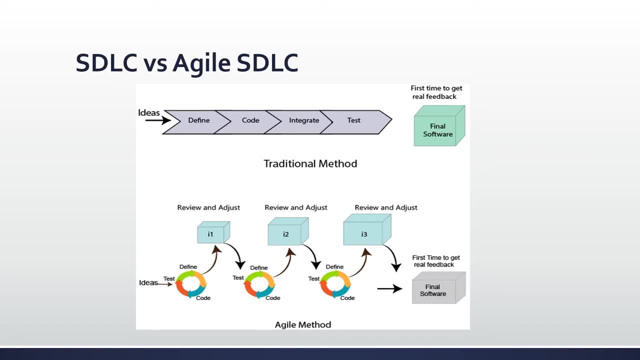 it is difficult to estimate the resources and developmental costs. The Agile SDLC process flow starts with a concept, which the projects are imagined and prioritized. the inception, which is where team members are created, funding is put into place and basic environments. 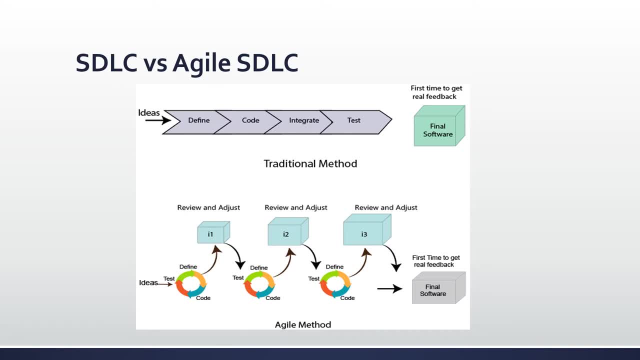 and requirements are discussed. Iterations, which is where the software development team works to deliver working software is based on a requirement and feedback. The release, which is perform quality assurance or QA testing and provides internal and external training, documentation, development and final version of the iteration in the product. And then 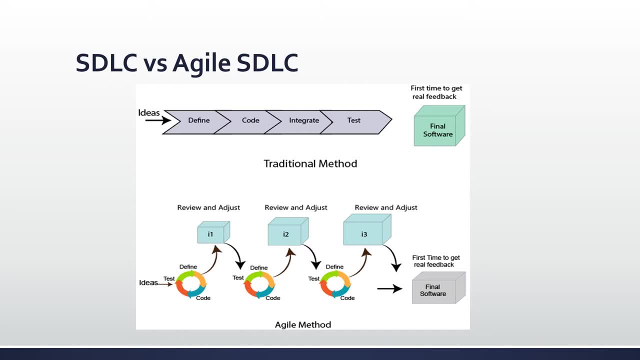 finally, production and its ongoing support of the software. The Agile SDLC model is designed to deliver a high-quality, high-performance, high-performance software. The Agile SDLC model is designed to deliver a high-performance, high-performance, high-performance software. So what is Agile methodology? An Agile methodology? 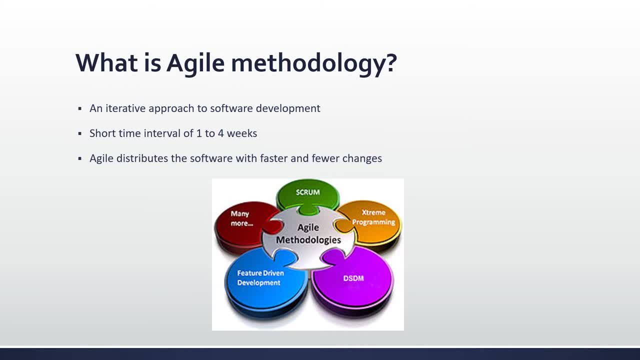 is an iterative approach to software development. Each iteration of Agile methodology takes a short time interval of one to four weeks. The Agile development process is aligned to deliver the changing business requirements and it distributes the software with faster and fewer changes. In a single-phase software development usually takes about six to 18. 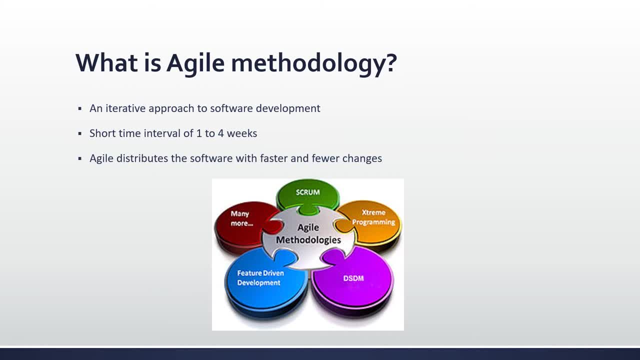 months In a single-phase development. all the requirements gathering and risk management factors are predicted initially up front. The Agile software development process frequently takes the feedback of workable product and the workable product is delivered within one to four weeks of an iteration. 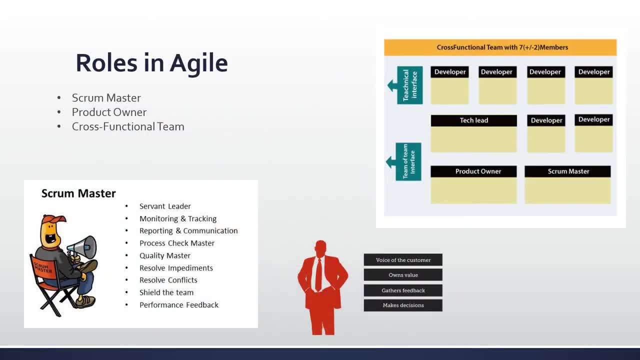 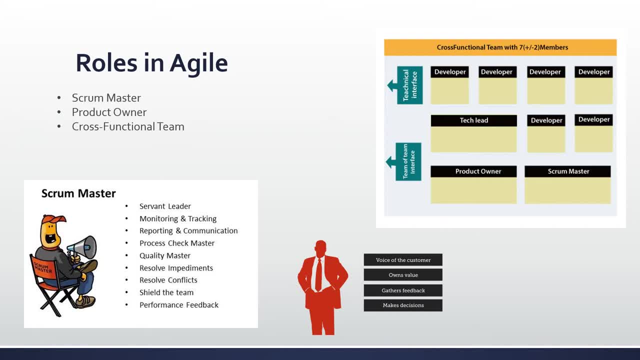 The Scrum Master is a team leader and facilitator. The Scrum Master is a team leader and facilitator. This team leader can be a team leader and facility provider who helps the team members to follow Agile practices so that the team members meet their commitments and customers. 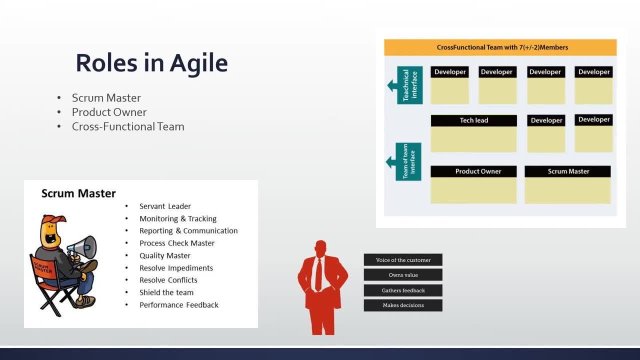 requirements. The Scrum Master plays the following responsibilities: They enable the close cooperation between all roles and functions. They remove all the blocks which occur. They safeguard the team from any disturbances. They work with the organization to track the progress and processes of the company. 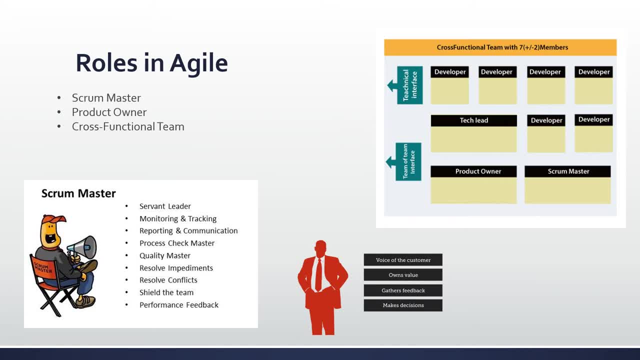 They ensure that Agile inspectors are motivated to monitor all processes in professional use. They ensure that Agile inspectors are motivated to monitor all processes in professional use and adapt. processes are leveraged correctly, which includes planned meetings, daily stand-ups, demos, reviews, retrospective meetings and facilitating 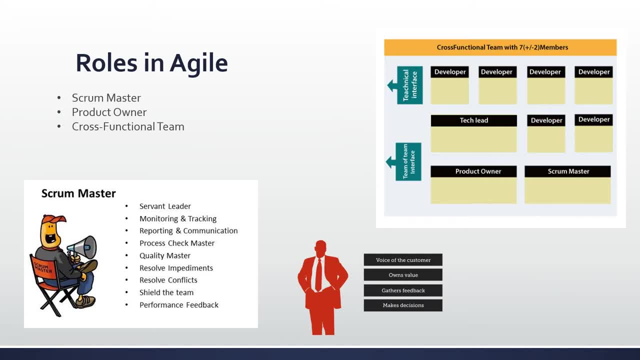 team meetings and decision-making processes. The product owner is one who runs the product from a business perspective. The product owner plays the following responsibilities: He defines the requirements and prioritizes their values. He sets the release dates and contents. He takes an active role in 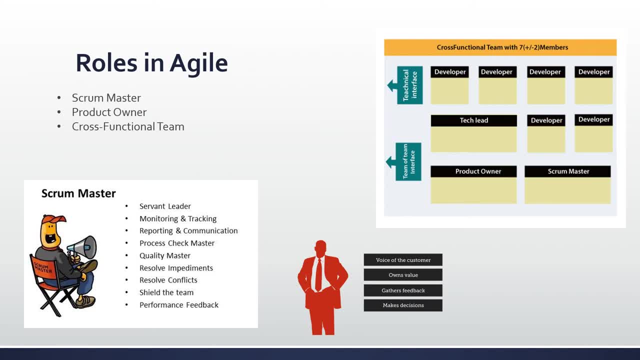 iteration and release planning meetings. He ensures that the team is working on the most valued requirement. He represents the voice of the customer. He accepts the user stories that meet the definition of done and defined acceptance criteria And the cross-functional team. Well, every Agile. 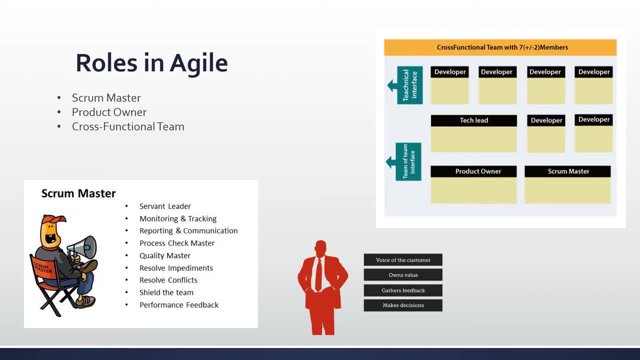 team contains self-sufficient teams with about five to nine teams per team, And the cross-functional team. Well, every Agile team contains self-sufficient teams with about five to nine members. The average experience of each member usually ranges between six to ten years. The 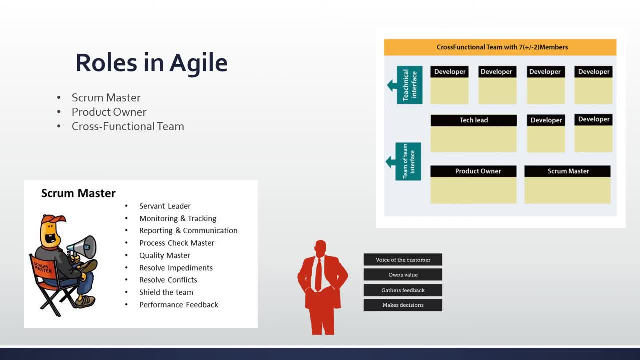 Agile team consists of three or four developers, at least one tester and one technical lead, one scrum master and one product owner. The scrum master and product owners are considered as part of the team interface, so, on the other hand, remaining members are part of the technical 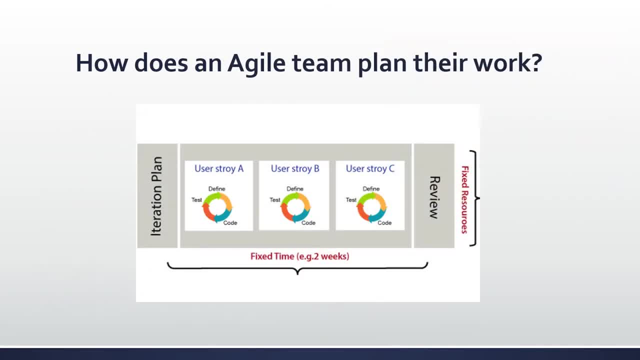 interface. How does Agile teams plan their work? An Agile methodology is not a specific set of ceremonies or specific development techniques. rather, it is a group of methodologies that demonstrate a commitment to tight feedback cycles and continuous improvement. An Agile team works in iterations to deliver the customer requirement, and each iteration takes 10 to 15 days. However, 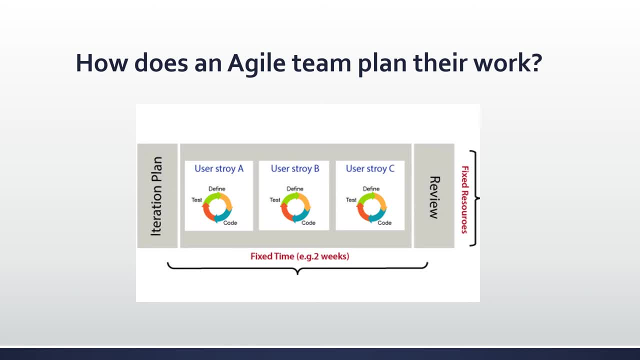 the original Agile team is only required to meet the requirements of the Agile team to improve its Agile manifesto didn't set the time period of two-week iterations or an ideal team size. Each user requirement is a planned based and their backlog prioritization and size. The team decides how much scope they have and how many. 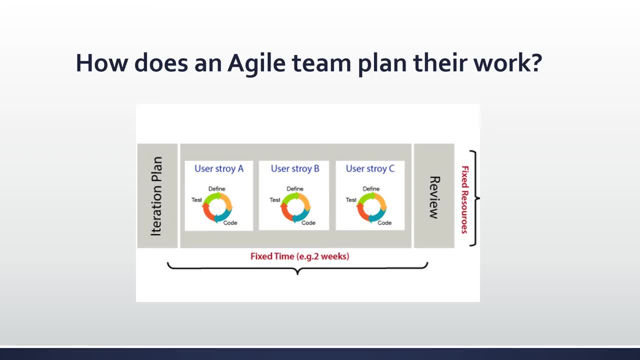 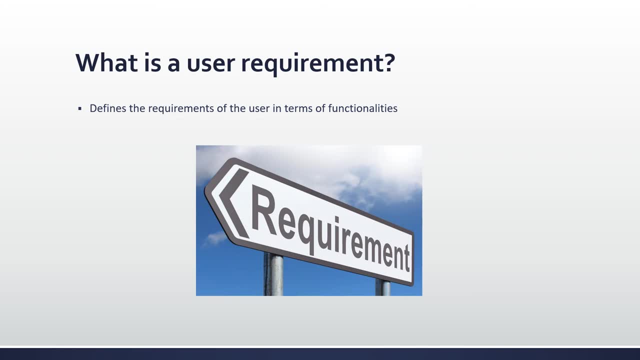 hours available, with each team to perform their planned tasks. What is a user requirement? The user requirement defines the requirements of the user in terms of functionalities. There may be different types of functionalities. It could be a user role, such as: I want certain functionality so that whatever. 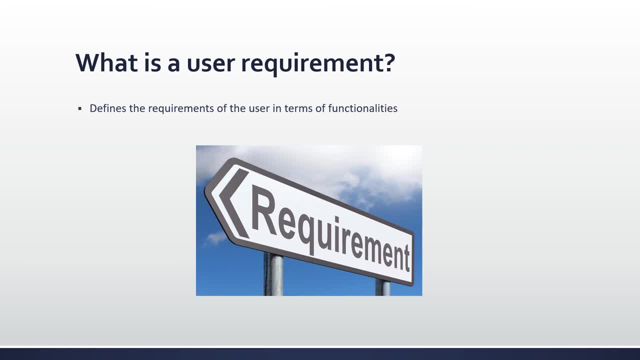 the business value is or it could be. in order to whatever the business value is, as a user role, I want whatever functionality. During software release planning, a rough estimate is given to a user requirement using relative scale points and during iteration planning, the requirement is broken down into. 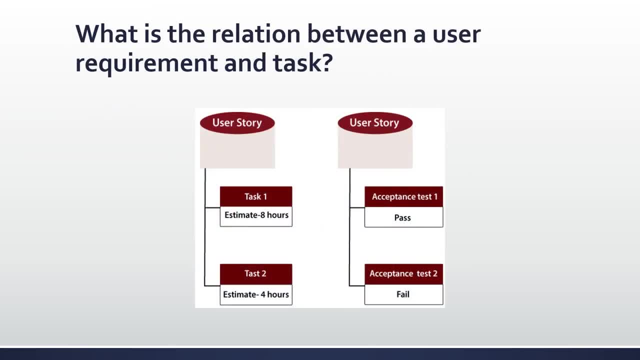 tasks. So let's now talk about the relation between user requirements and tasks. User requirement talks about what is to be done. It defines the needs of users. Tasks talk about how it is to be done. It defines how functionality is implemented. User requirements are implemented by tasks. 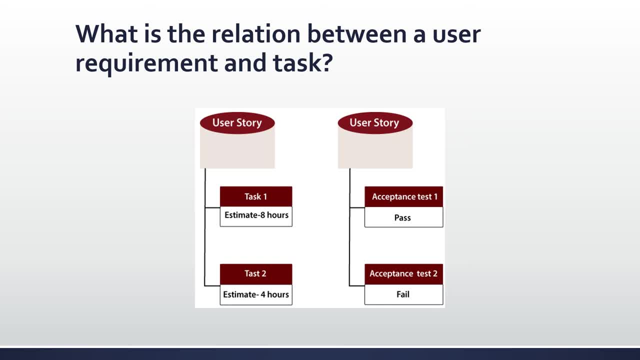 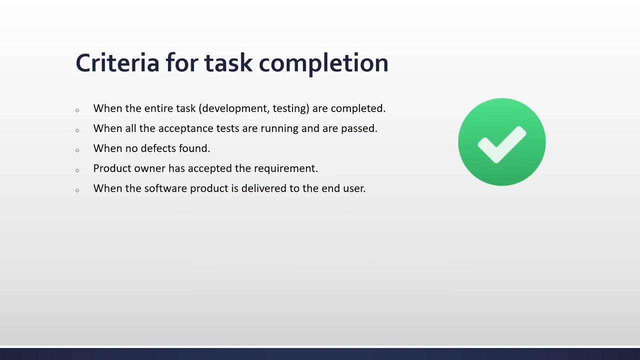 and every requirement is gathered as a task. User requirements are divided into into different tasks, when it is planned. in the current iteration, user tasks are estimated in hours based, generally between 2 to 12 hours. requirements are validated using acceptance testing the criteria for task completion. then the agile team decides when, what the meaning of the task.